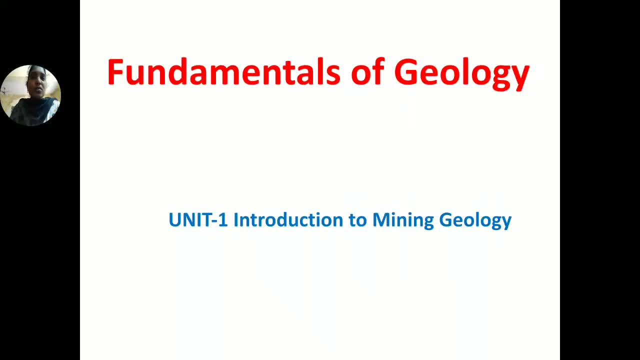 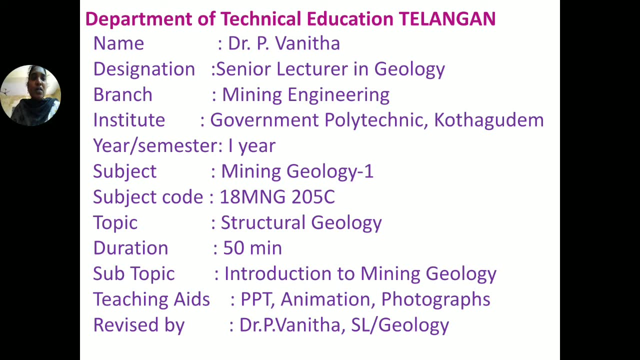 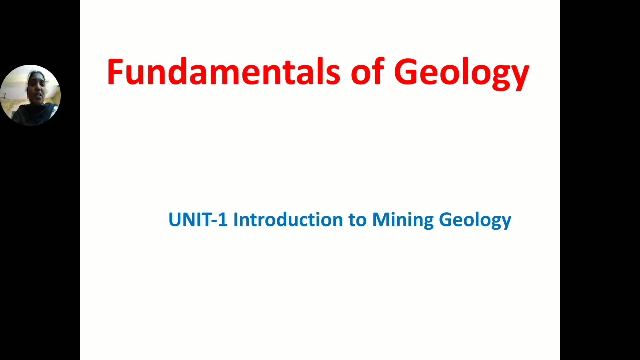 Good morning to all. My name is PVanitha, Senior Lecturer in Geology, Government Polytechnic Kottagudam, In Mining Branch. one subject is Mining Geology ie- Fundamentals of Geology in 1st Chapter, Introduction to Mining Geology. 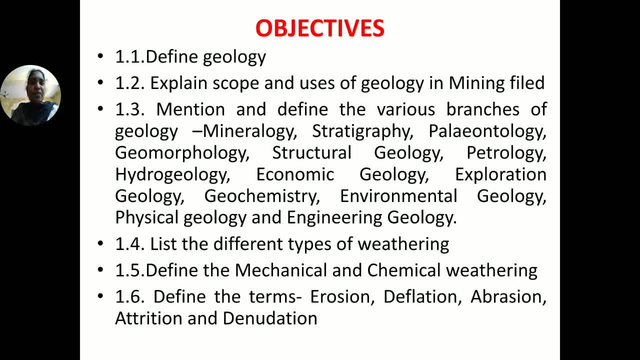 Objectives of Geology: 1.1. Define Geology. 1.2. Explain Scope and Uses of Geology in Mining Field. 1.3. Mention and Define the Various Branches of Geology: Mineralogy, Stratigraphy, Paleontology, Geomorphology, Structural Geology, Petrology, Hydrogeology, Economical Geology, Exploratory Geology. 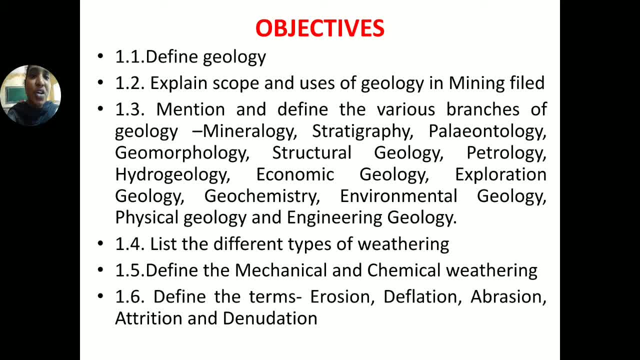 Geohemistry, Environmental Geology, Physical geology, Engineering Geology- 1.4.. List the different types of weathering: 1.5.. Define Mechanical & Chemical Weathering: 1.6.. Define Terms like Erosion, Deflation, Abr bermans, comm常, Abrietian, De-nudation and Attrition. 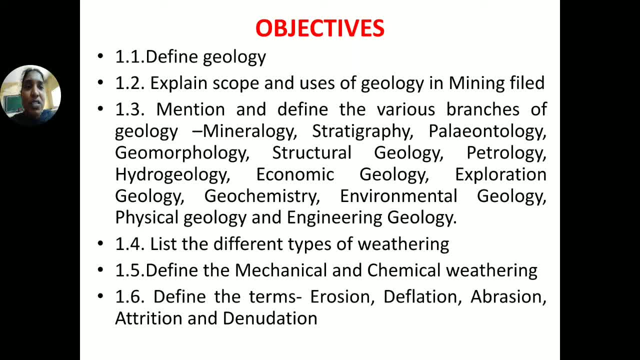 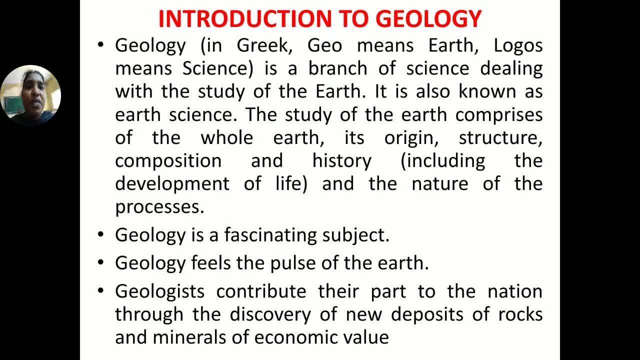 introduction to mining geology. first chapter objectives. introduction to geology. what is geology? why we studying in mining engineering students? why to learn geology. it is the science subject geology word in greek word. in the greek geo means earth, logos means science- is a branch of science dealing with the study of the earth, it. it is also known as: 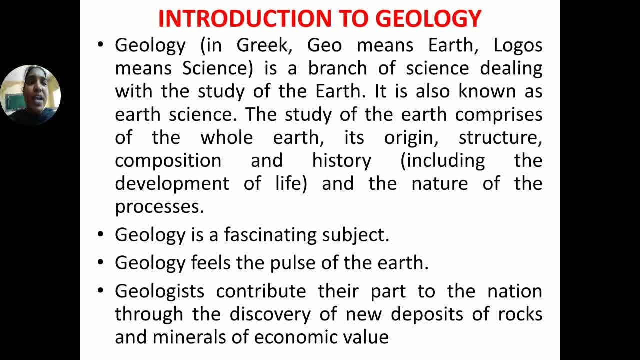 earth science: the study of the earth, compressing of the whole earth, it origin, structure, composition and history, including the development of life and the nature of the process. it is all over studied. the earth science that, including all structures, origin, composition and history, all over topographical features studied: the 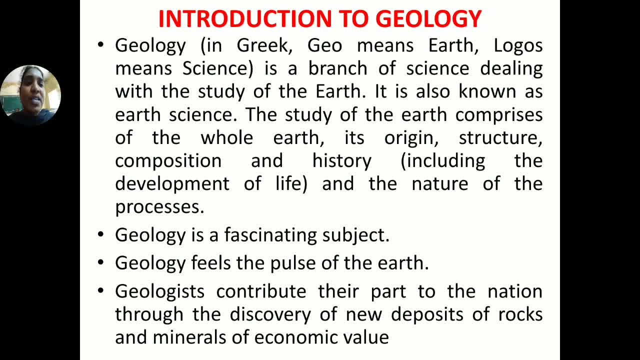 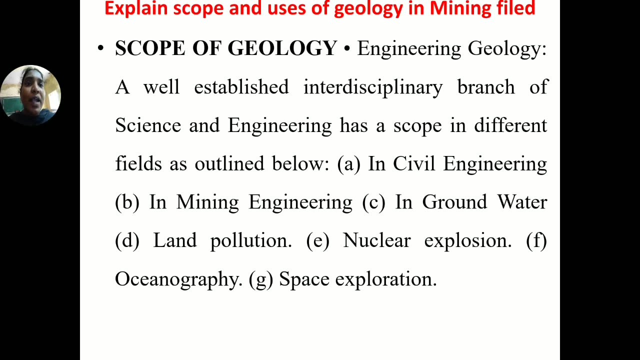 in geology. geology. geology is a fantastic subject. geology feels the pulse of the earth. geologist contributes their parts of the nation through the discovery of new deposits of rocks and minerals, and economic values, and explain the scope and uses of geology in mining field. 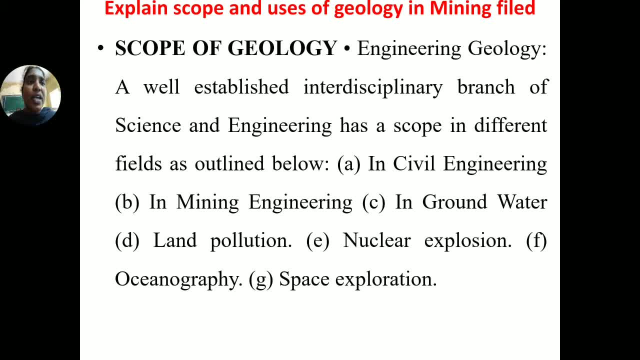 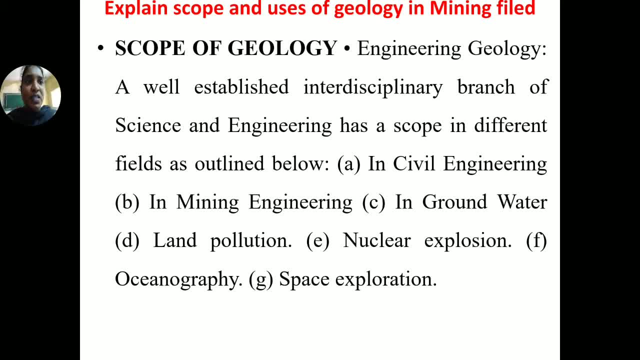 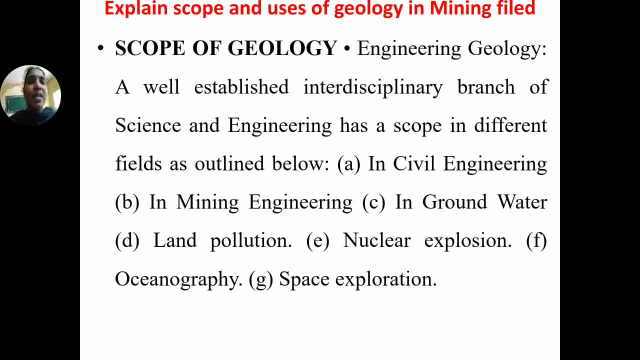 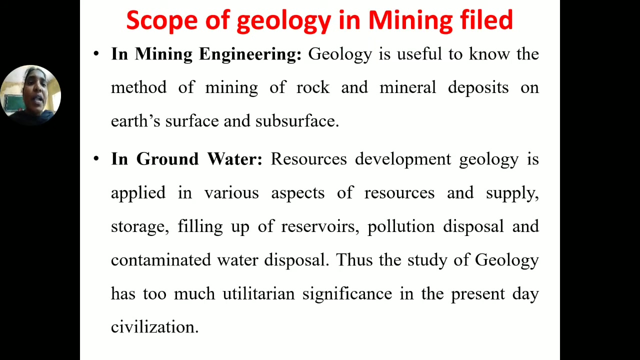 that means us, and and lead, that means and drastic, and it um well established and cinq five. so A In Civil Engineering and B Mining Engineering, C In Groundwater and Land Pollution, E- Nuclear Explosion, F- Oceanography, G- Space Exploration And in Mining Engineering. what is the scope of in Mining field? 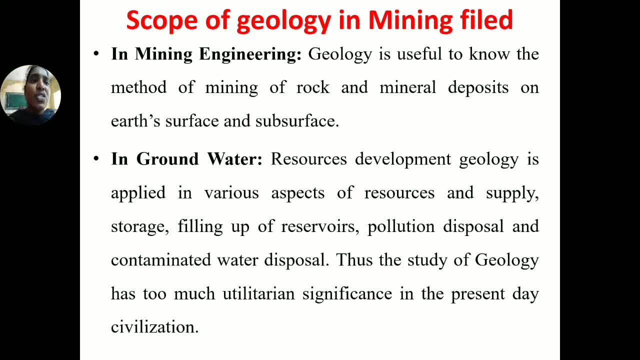 In Mining Engineering Geology is useful to know the method of mining of rock and mineral deposits on earth surface and subsurface, Mainly rock and mineral deposits. how to identify, how to excavation, how to exploration of the surface and subsurface in the ground. 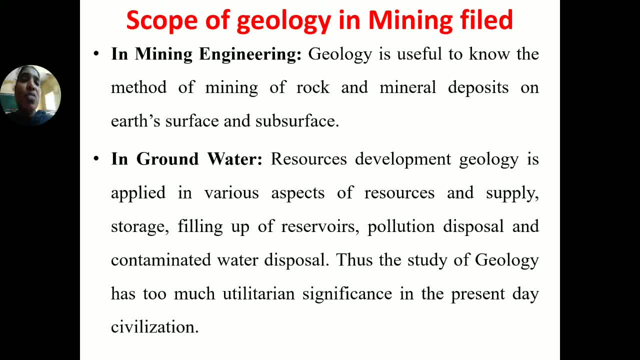 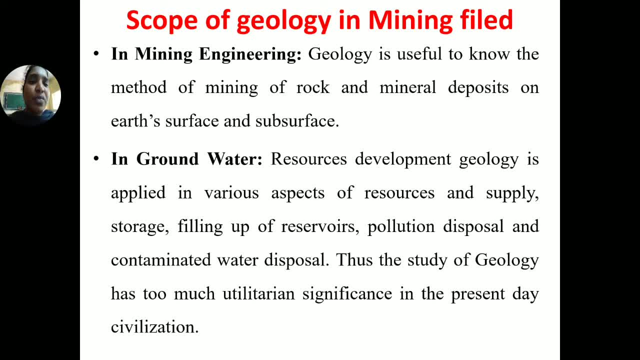 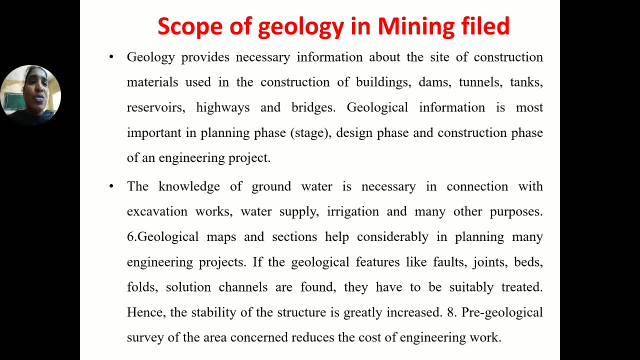 And pollution, disposable and different type of water resource. These are in study in Groundwater. Thus, the study of Geology has too much utilitarian significance in the present day civilization. And also Geology provides necessary information about the site of. And also Geology provides necessary information about the site of construction materials used in the constructions of buildings, dams, tunnels, tanks, reservoirs, highways and bridges. 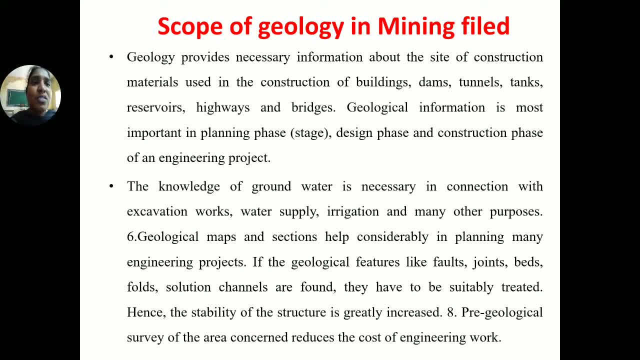 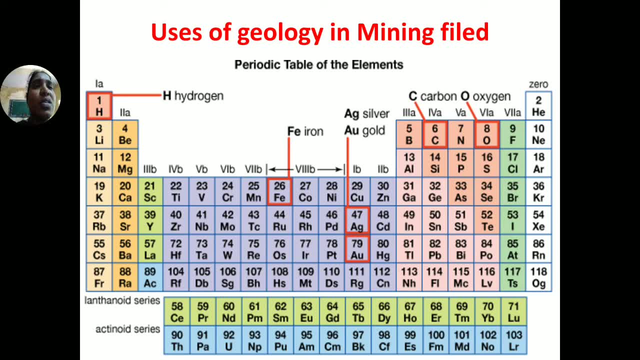 In Geology: geological information is most important in planning phase stage design. In Geology: geological information is most important in planning phase stage design rocks. so that's why uses of in mining field very useful in so much minerals and rocks and elements. 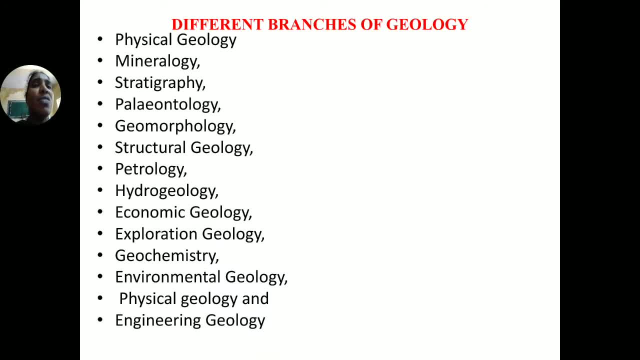 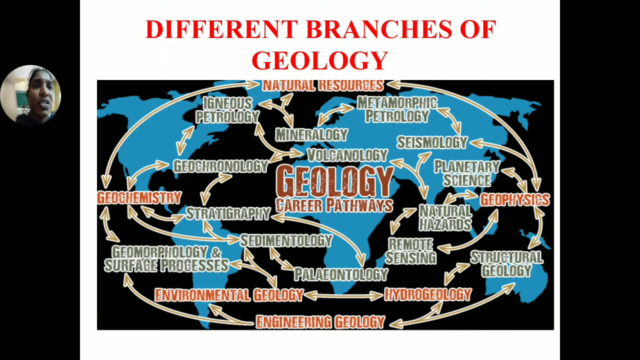 and different branches of geology. these are physical geology, mineralogy, stratigraphy, paleontology, geomorphology, structural geology, petrology, hydrogeology, economic geology, exploration geology, geochemistry, environmental geology, physical and engineering geology and different branches of geology, natural resource and some metamorphic igneous petrology. 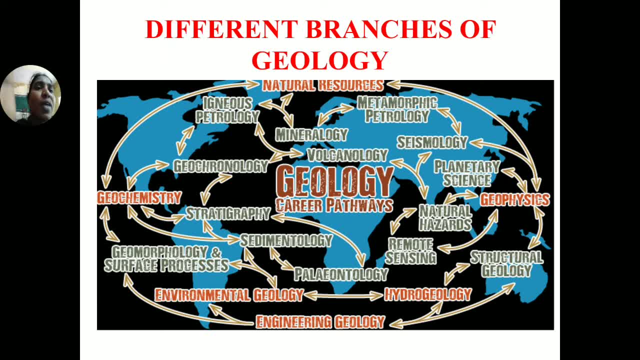 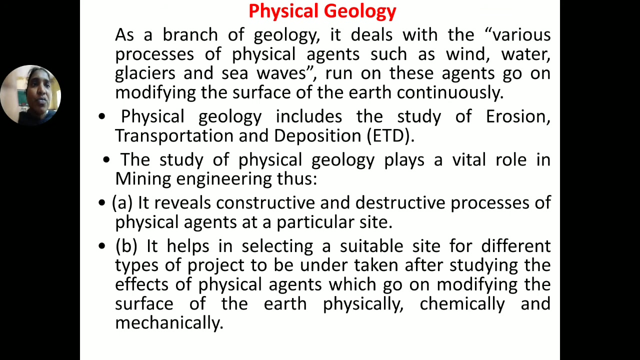 and some mineralogy, vulcanization and metamorphic petrology, seismology, paleo, and, and, and, and, and, and, and. in geological field and speaking geology has a branch of geology. It deals with the various process of physical agents such as wind, water, glaciers and sea waters. Run on, these agents go on, modify the surface. 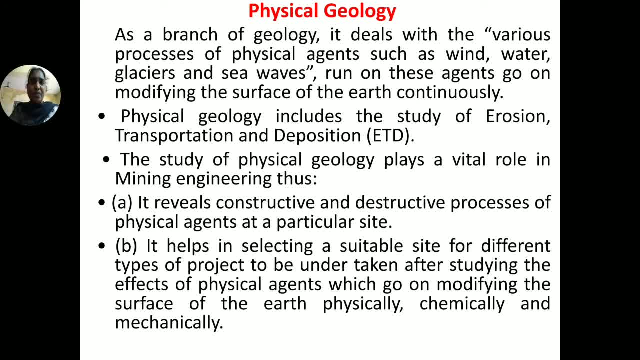 of the earth continuously, Nothing but physical geology. it is various process, physical agents and physical geology include the study of erosion, transportation and deposition. The study of physical geology plays a vital role in mining engineering. It reveals constructive and destructive process of physical 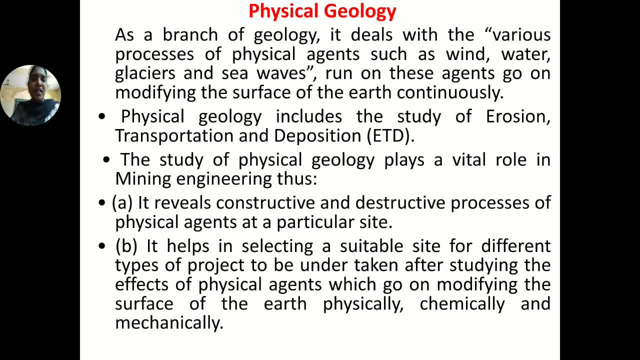 Agents at a particular site. It helps in selective and selective, a suitable site for different types of projects to be undertaken after studying the effect of physical agents which go on modify the surface of the earth: physical, chemical and mechanical- Mainly physical geology in process. 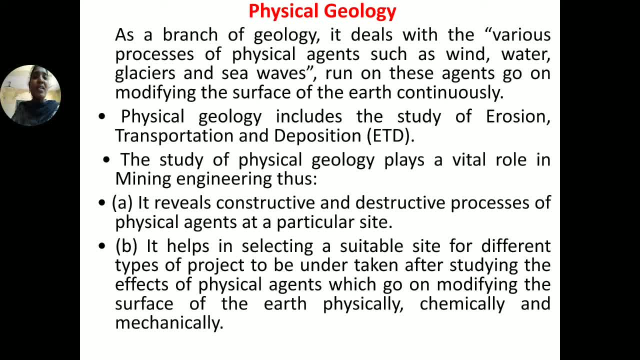 It includes analysis of natural processes and various process by physical agent- endo genetic and exo genetic process- due to change the its surface or earth movements and an earth sub-surface changes. It is called the physical geology Father of physical geology. James Hutton, Modern father of EEG actual. due to change the earth surface matters not only growth of the earth, but also the ancient earth, because the earliest geological giants still be alive. We, the human beings who have been living in unknown places, are born and 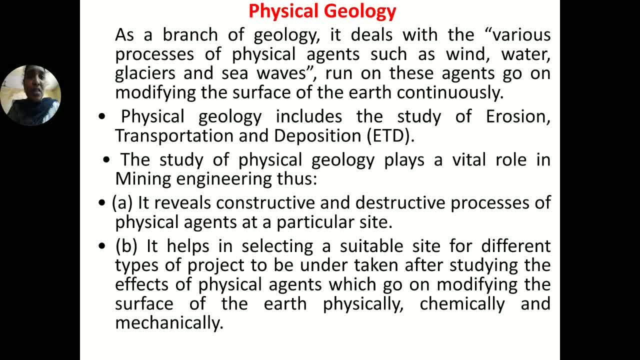 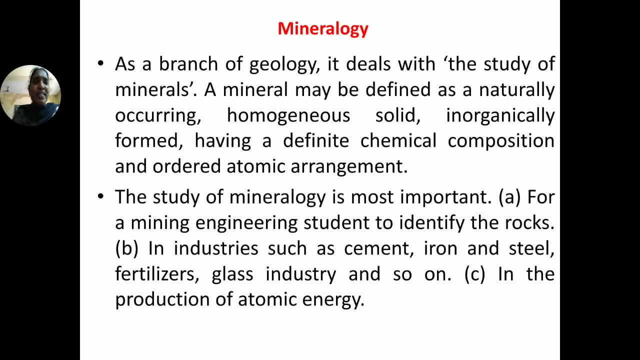 living on Earth. These changes came in order to change earth condition. if we go up and down talks, physical geology is james hurton and mineralogy as a branch of geology, it deals with the study of minerals. mineralogy deals with the study of minerals. a mineral may be defined as a naturally. 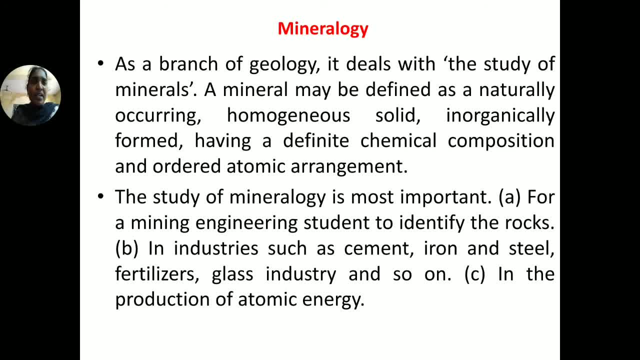 occurring homogeneous solid inorganically formed, having a definite chemical composition and ordered atomic arrangement. the study of mineral mineralogy is most important for a mining engineering student to identify the rocks, and also the study of mineralogy is the most important in industries such as cement, iron and steel, fertilizers, glass industries and so on. 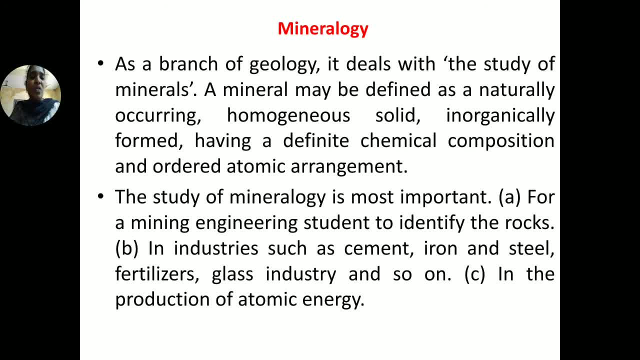 and also, most important in my mineralogy, in the production of atomic energy. these are minerals. mineral is the study, study of minerals, nothing but mineralogy. mineral it occurring homogeneity, homogeneous substance, solid, inorganically formed, having a definite chemical and atomic arrangement. physical properties and the chemical properties and the atomic arrangement. 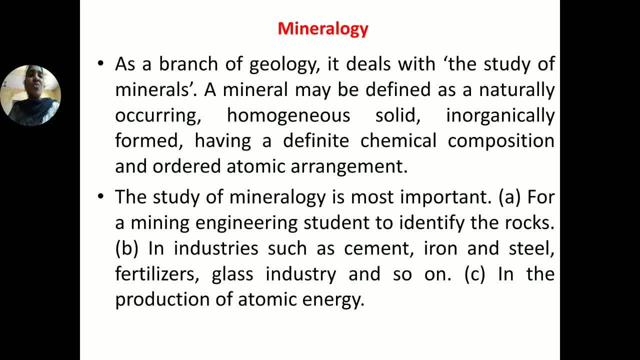 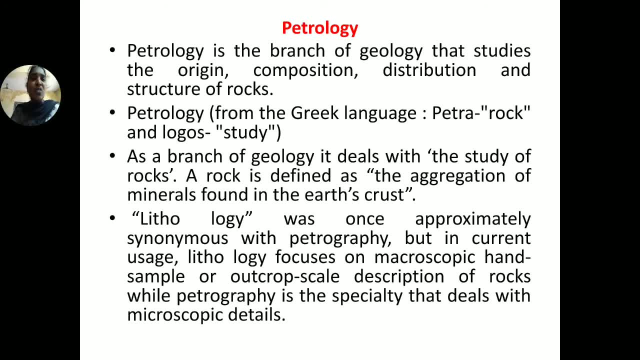 is called the mineral. these total deals with the mineral geology and the petrology. petrology is the branch of geology that studies the origin, composition, distribution and construction of rocks. petrology- from the greek language petro means rock and logos means study- as a branch of geology is. 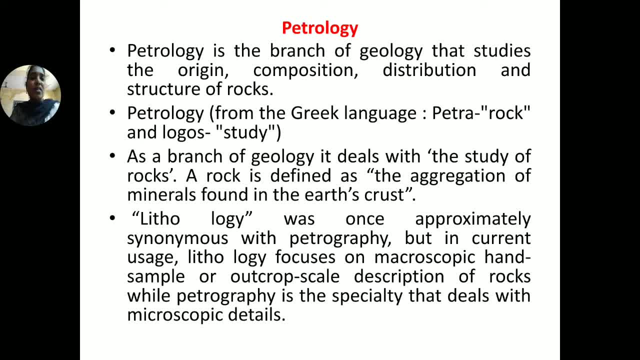 it is deals with the study of rocks. a rock is defined as the aggregation of minerals found in the earth crust. lithology was once approximately synonyms with petrography, but in current usage lithology focuses focus on microscopy, hand sample or outk Bakks scale description of rocks, while petrography is the. 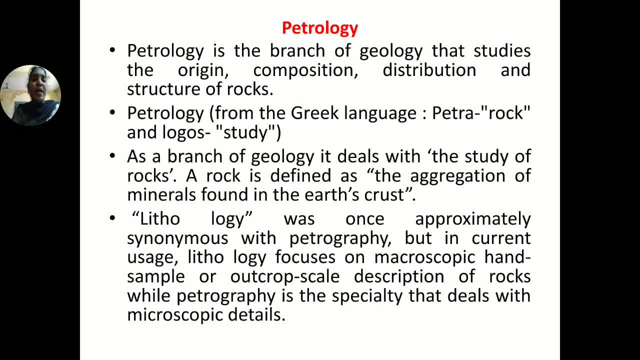 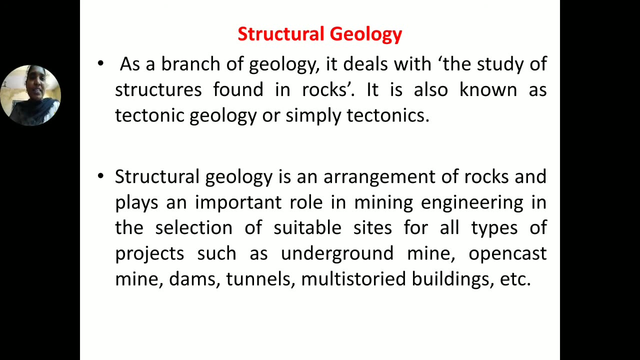 specially that deals with the microscopic details, patients of the near зам箭 study of rocks. petro means rock, logos means study rocks, composition rocks, origin rocks, distribution rocks. it uses structures, structures. it deals with the petrology and structural geology As a branch of geology. 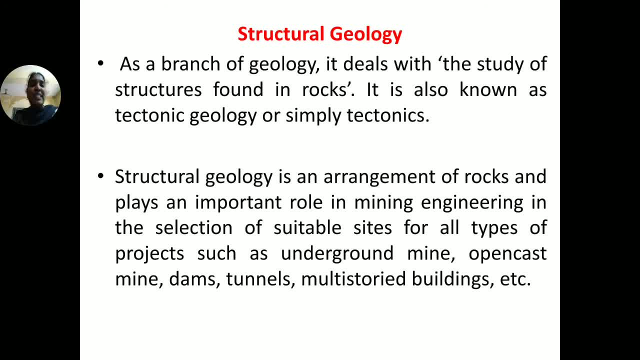 it deals with the study of structures found in rocks. It is also known as tectonic geology or simple tectonic Structural geology is an arrangement of rocks and plays an important role in mining engineering in the section of suitable sites for all type of projects. 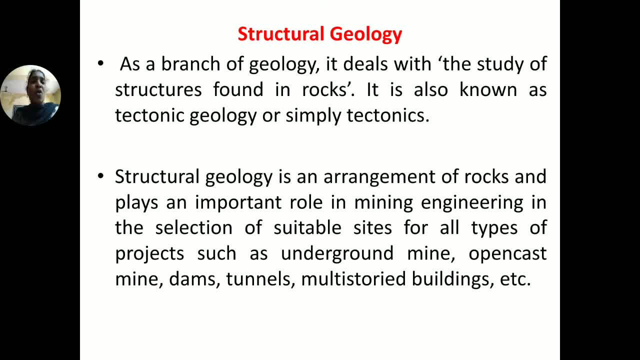 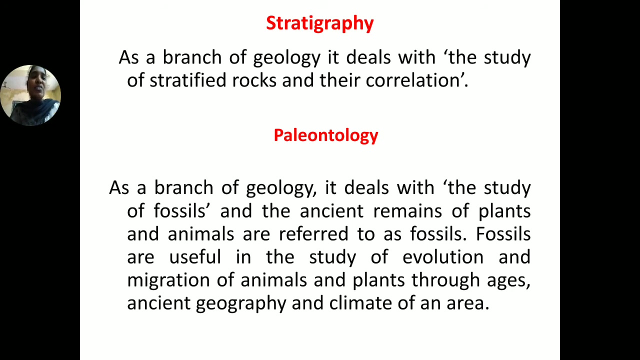 such as underground mine, opencast mine, dam tunnel, multi-store building that is, etc. Structural geology is known as architectures of rocks or rearrangement of reconstruction of the rocks. that is known as structural geology and stratigraphy as a branch of geology. it. 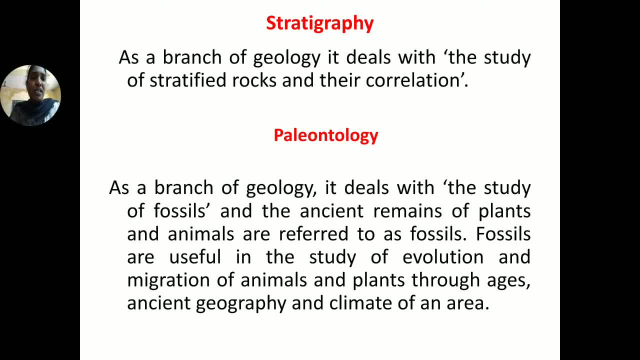 deals with study of stratified rocks and their correlation History of a rock, or study of a solid or round rocks or rocks and intersected rocksau. Lum Privateopf envie au revoir of strata or layers of the bedrock. nothing but stratigraphy. Strata means layer graphy. 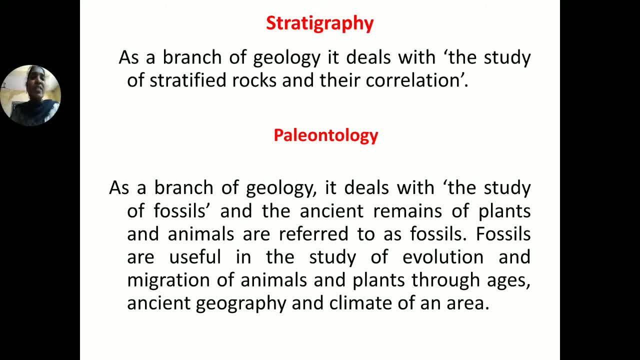 means description. It deals with the layer of rocks, stratified rocks and paleontology. As a branch of geology. it deals with the study of fossils, and the instant remains of plants and animals are referred to as fossil. Fossils are useful in the study of evolution. 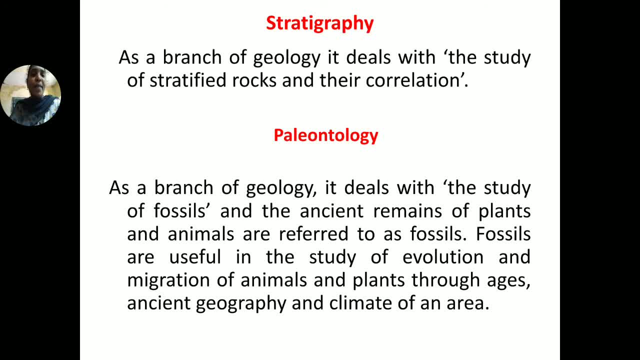 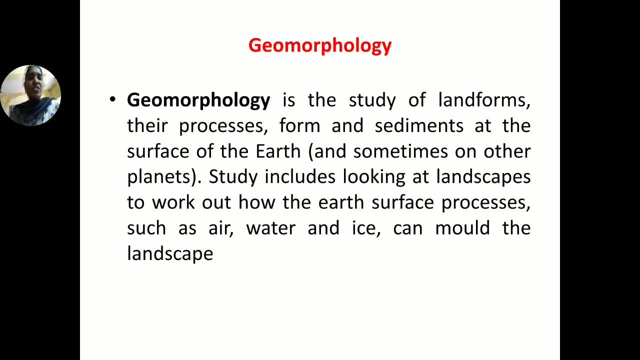 and migration of animals and plants through ages and instant geography and climate engineering of an area In particular area. paleontological data- it is useful- of rock time or bed, previous data And geomorphology. geomorphology is the study of landforms, their process from. 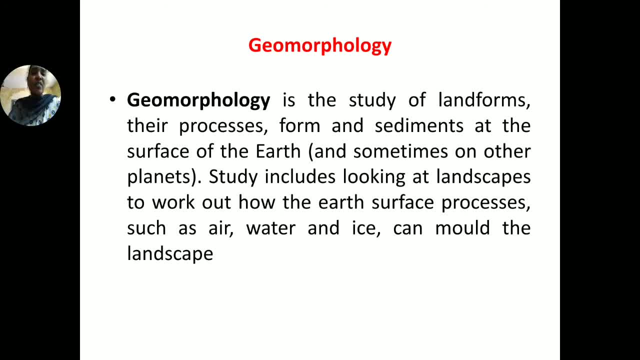 and sediments at the surface of the earth and sometimes on other planets. Study includes looking at landscapes to work out how the earth's surface process, such as air, water and ice, can mold the landscape. Geomorphology studied the land surface to change the air. 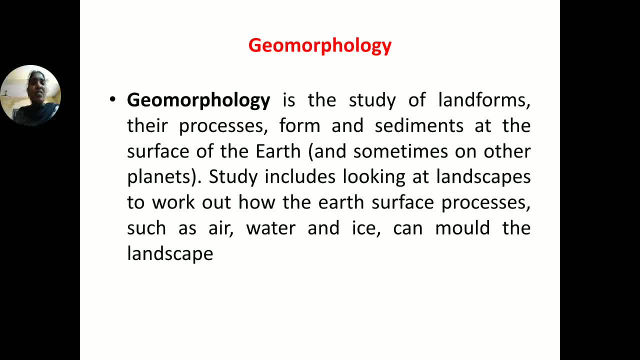 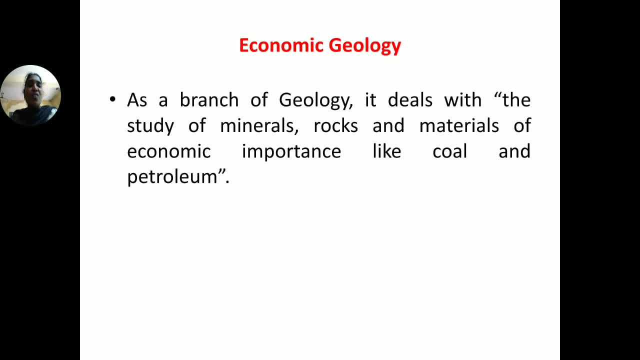 surface Earth are process of sediments to change the surface of the earth. It is study of geomorphology And economical geology. as a branch of geology it deals with the study of minerals, rocks and materials of economic importance like coal and petrol. 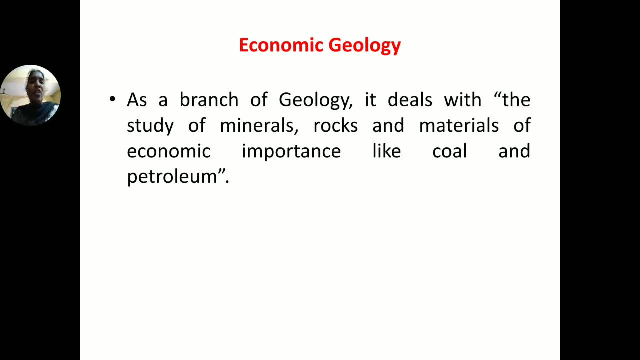 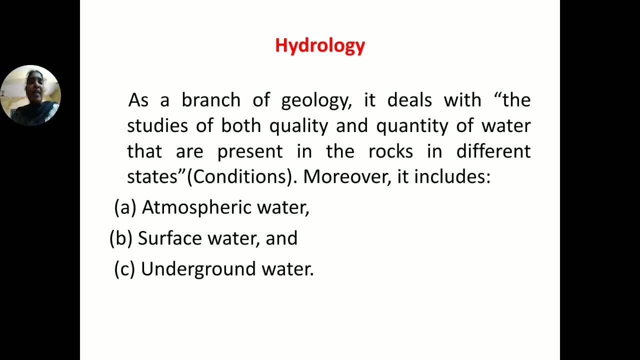 These are useful in mankind. Economical geology is very useful in our nation. Hydrology. as a branch of geology, it deals with the study of earth quality and quantity of water that are present in the rocks in different states conditions. Moreover, it includes atmospheric water, subsurface water. 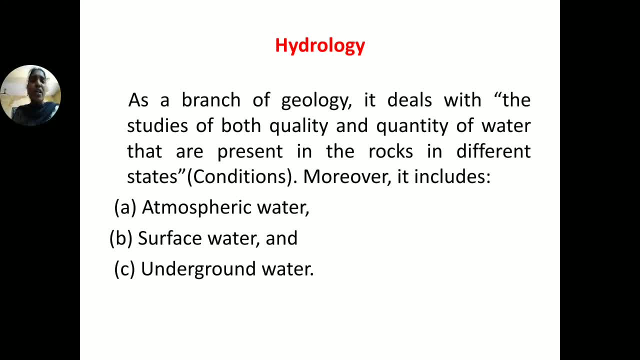 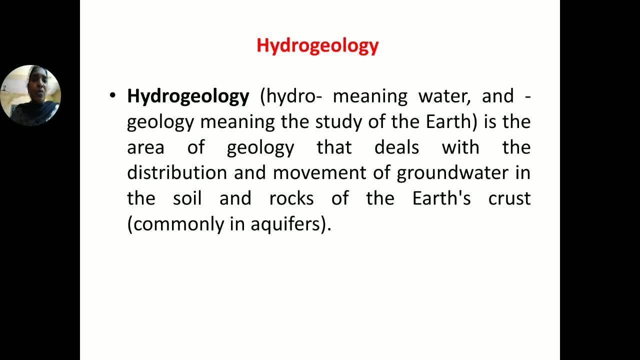 Under ground water. These are very studied. hydrogeology- Hydro means water and geology means the study of earth- Is the area of geology that deals with the distribution and movement of ground water in the soil and rocks of the earth's crust. 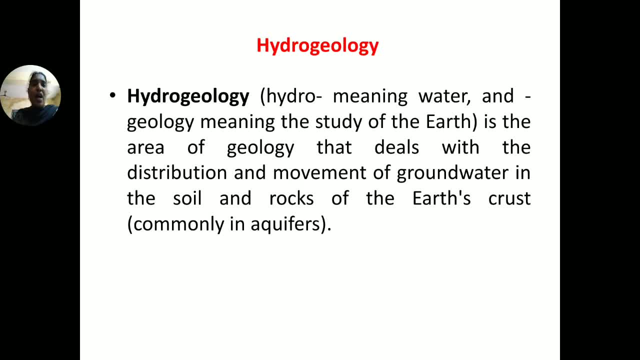 Commonly in Hydrology means water and geology mean study of earth. It particular rocks area, particular ground, earth surface area distribution. how much is water quality? aquifer is present, how much water is there? it is studied in hydrogeology. 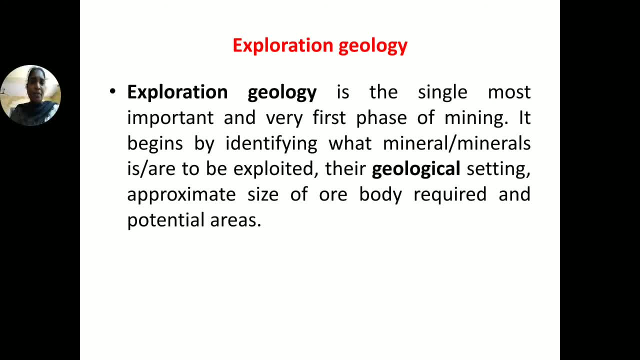 And exploration geology. Exploration, Exploration Geology is the single most important and very first phase of mining. It begins by identifying what minerals are to be exploited, their geological setting, approximate size of ore body required and potential areas. It is useful for mining engineering. 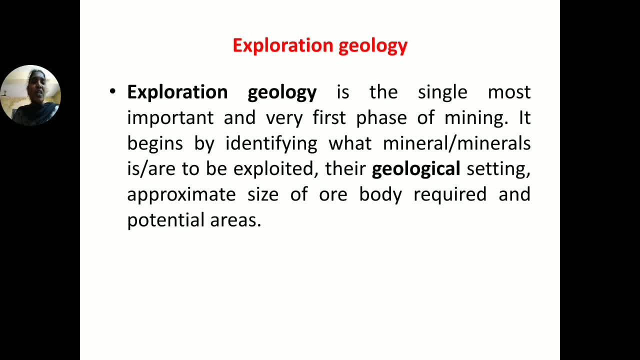 In exploration geology. It is used for minerals identification and rocks identification. that is, geological setting: approximate size, how much quality and quantity of the rocks, how size of ore body required in the potential area. It is total covered in exploration geology. 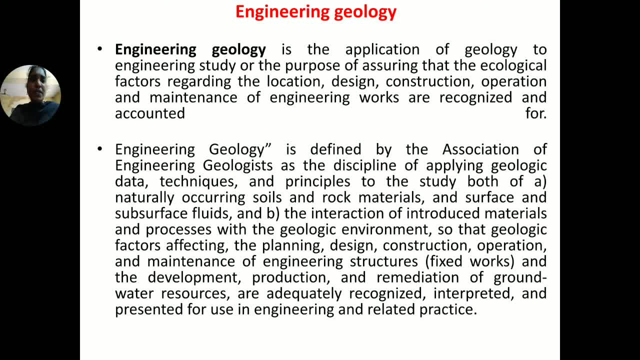 And last one, Engineering geology. Engineering geology. Engineering geology is the Application of the geology to engineering, study or purpose of assume that ecological factors regarding the location, design and construction, operation and maintain of engineering works. These are mostly useful of the our engineering. 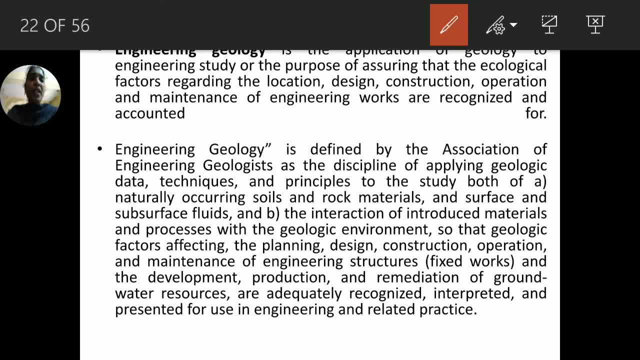 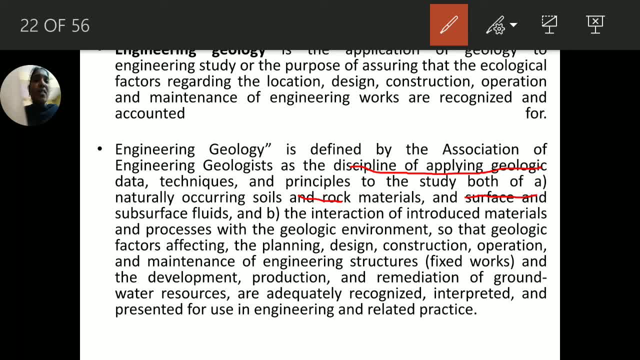 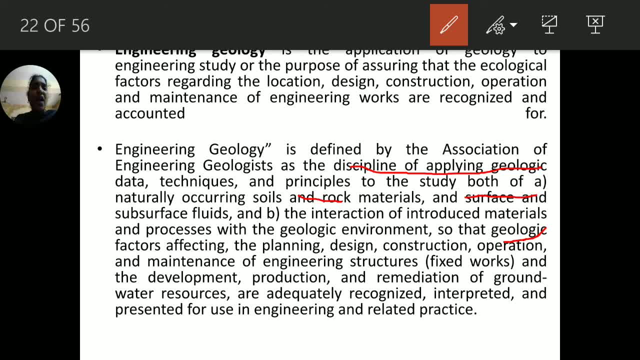 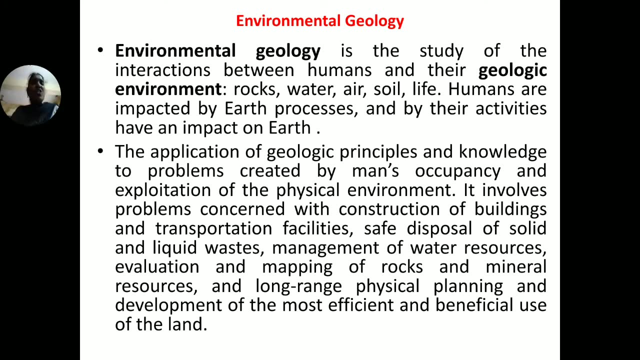 of groundwater resource are adequately recognized, interpreted and presented for us in engineering and related practice. Environmental geology is the study of the interaction between human and their geological environment: rocks, water, air, soil, life- these are geological environment. humans are. 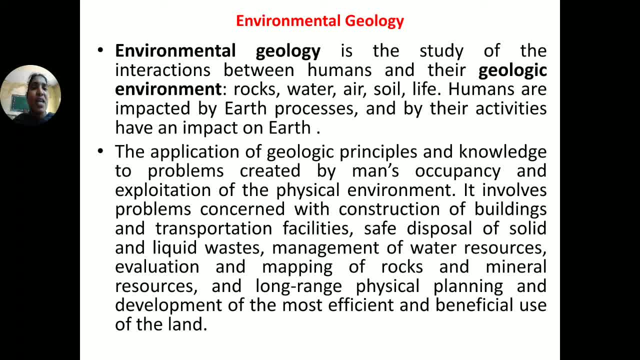 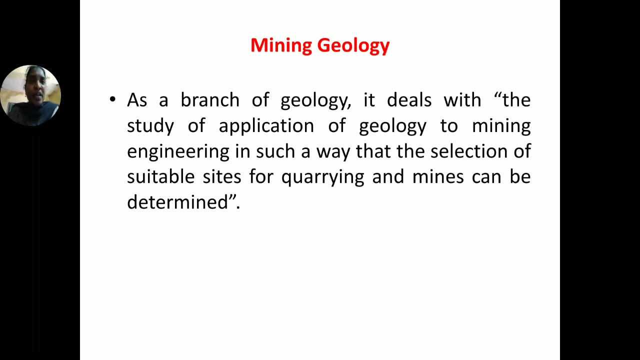 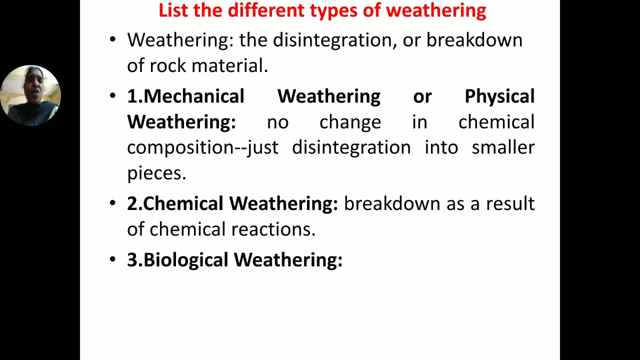 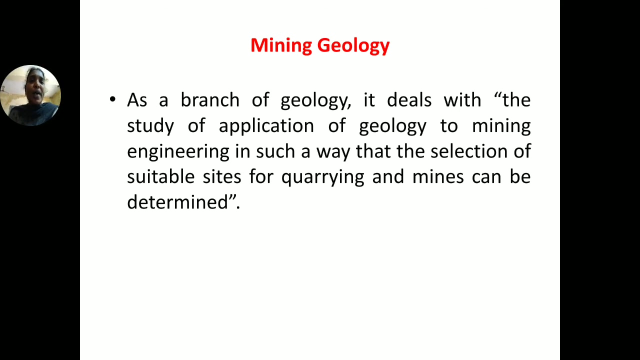 also geological environment. And last one, mining geology As a branch of geology. it deals with the study of application of geology to mining engineering.